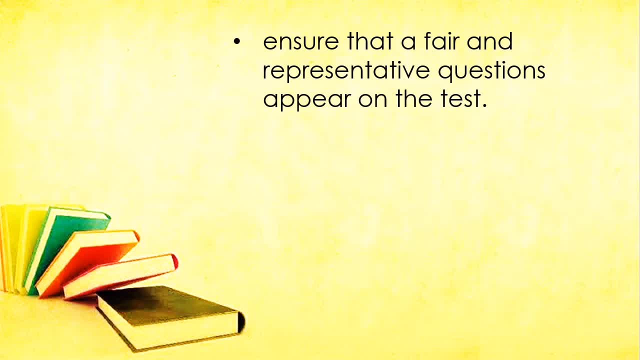 All questions are focused there. For example, we have 50-item test. Half of it are focused only on one content. We have measured each content, but how about the other tones? With TOS, the distribution of the number of test questions becomes fair. 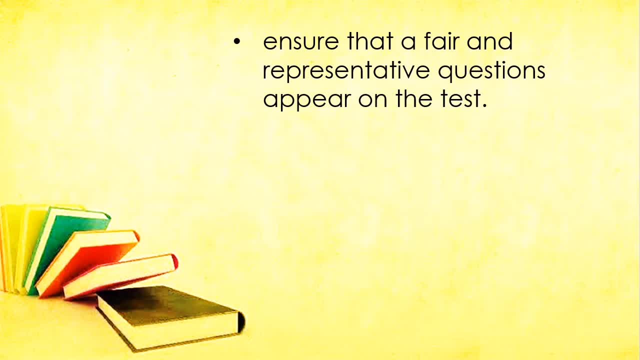 based on the length of hours taught to all learners compared to the number of intro and eyeliners constructed. Next, It improves the validity of the teacher's assessments based on the test constructed With TOS. test questions will bebstimulated, most of them airquez-sized. 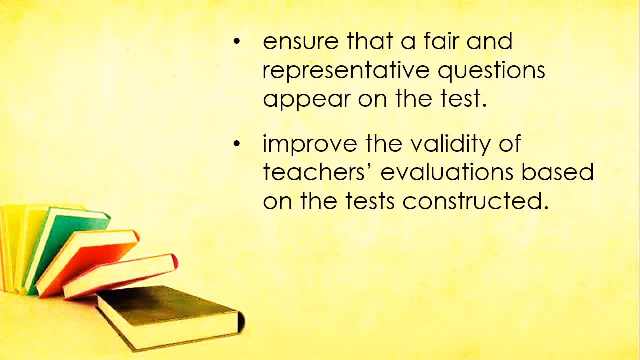 will be aligned with the learning objectives. Iko-consider mo lagi kung pasok ba yung questions sa skill na dapat matutunan ng students. It makes your evaluations more valid. It also helps teachers identify the type of items they need to include on their tests. 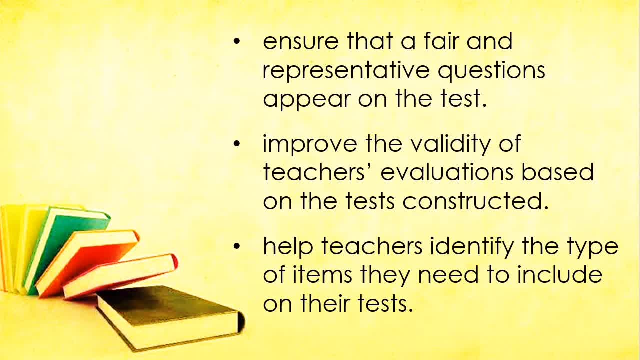 For example, if you think na yung questions na nagawa mo measured already a specific skill, mag-iisip ka naman ng test questions that could measure other learning skills. TOS also provides the teacher with evidence that a test has content validity. 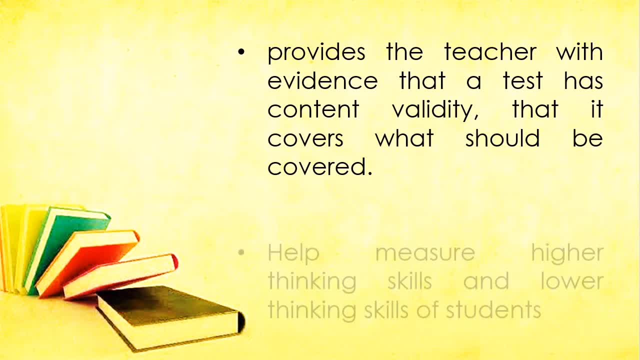 that it covers what should be covered and it helps measure higher thinking skills and lower thinking skills of students. The HATS question is important since this makes the bright students distinct from the rest of the class, Although there are instances during the exam, especially for some students. 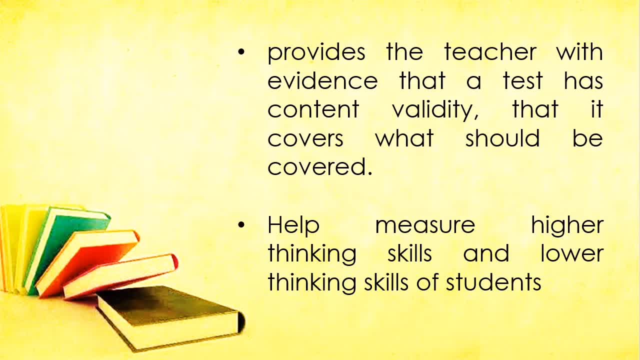 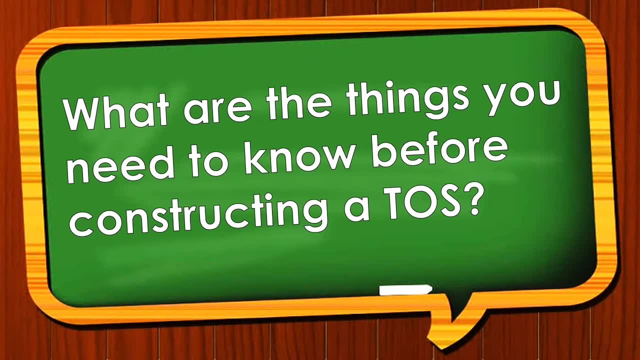 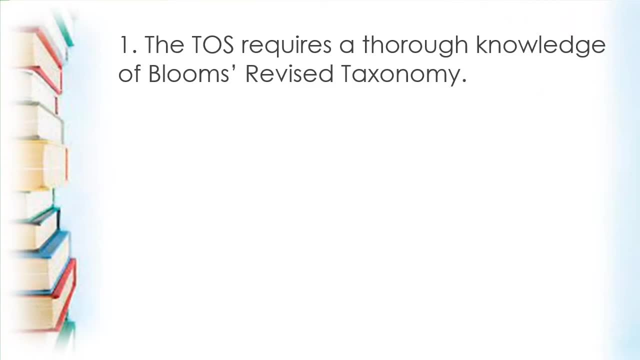 the most difficult questions in the test can be very easy, and there are also students who will find the easiest question difficult. Now what are the things you need to know before constructing a TOS? 1. The TOS requires a thorough knowledge of Bloom's Revised Taxonomy. 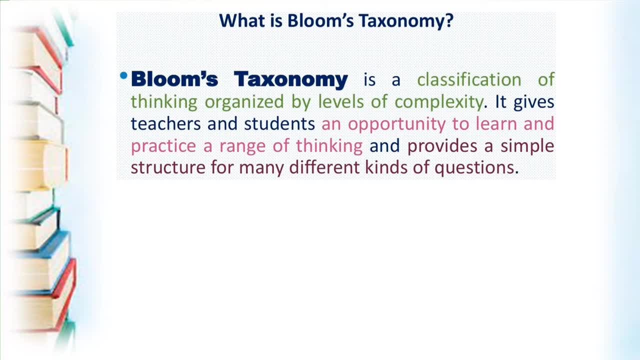 What is Bloom's Taxonomy? It is a classification of thinking organized by levels of complexity. We have the easy, average and difficult. It gives teachers and students an opportunity to learn and practice a range of thinking and provides a simple structure for many different kinds of questions. 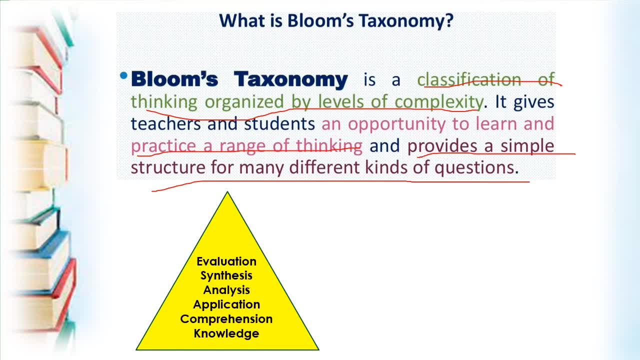 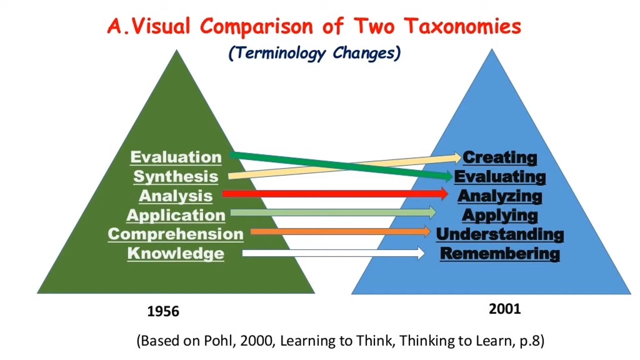 The 1956 Bloom's Taxonomy is a combination of taxonomy knowledge, comprehension, application, analysis, synthesis and evaluation. This was revised by Andersson and Crathwell in 2001 and used as a measurement tool for thinking. Here is the comparison of the two taxonomies, the 1956 and 2001.. 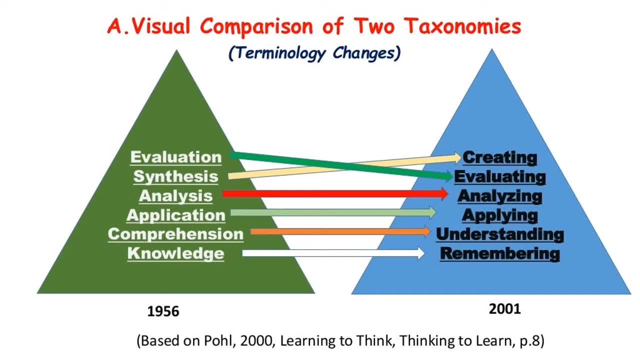 What do you notice? Noticeable is the terminology change. It is a combination of the two taxonomies. What is the terminology change? From knowledge to remembering, comprehension to understanding, application to applying, analysis, analyzing, synthesis, creating, evaluation, evaluating. 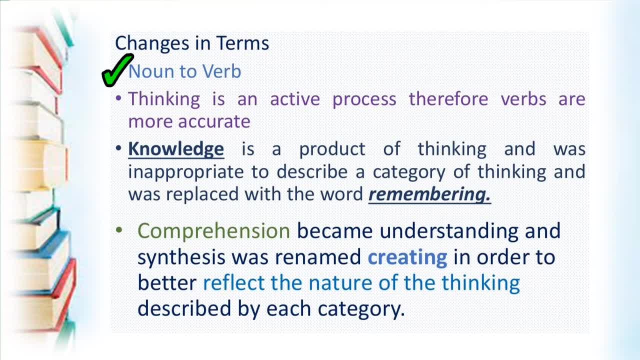 Why Changes in terms is from noun to verb. Thinking is an active process, Therefore verbs are more accurate. That's right. Knowledge is a product of thinking And was inappropriate to describe a category of thinking and was replaced with the word remembering. 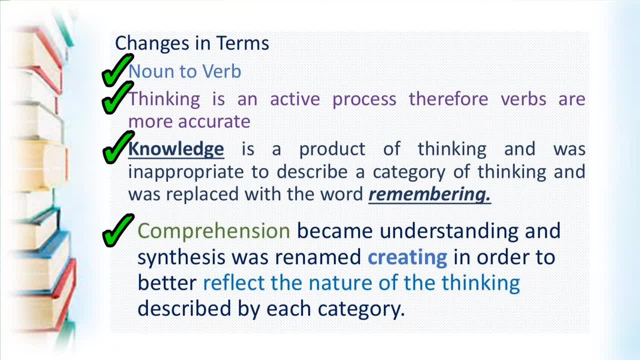 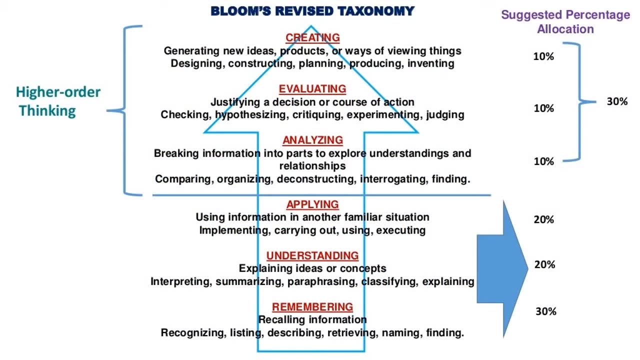 Comprehension became understanding and synthesis was renamed- creating, in order to better reflect the nature of the thinking described by each category. So those are the changes in terms. So here is the Bloom's Revised Taxonomy From level 1, we have remembering. 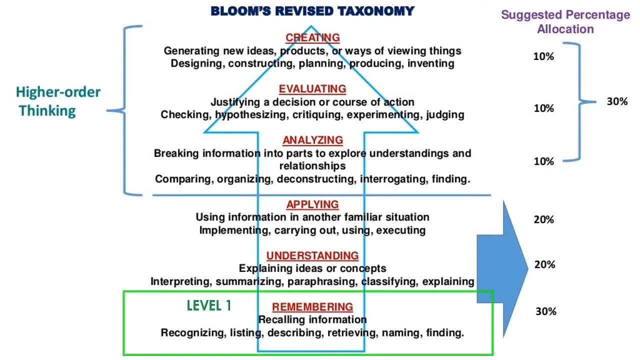 That is, recalling information. When your test question measures the recognizing, listing, describing, retrieving, naming, finding skill of the learners, That will fall under remembering More of like. as a teacher, you know which domain is measured by the questions you made. 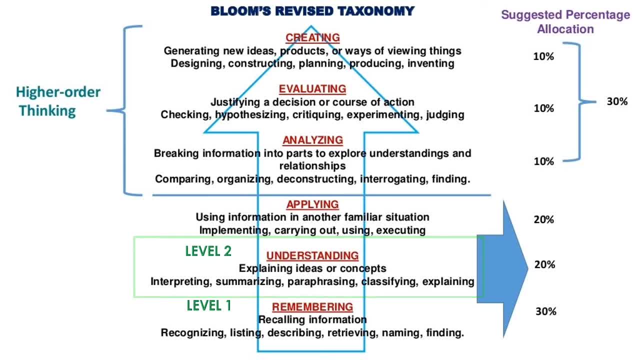 Level 2. Understanding Explaining ideas or concepts. When the test questions allow students to interpret, summarize, paraphrase, classify and explain. That is understanding. You measure students' comprehension- Level 3. Applying Using information in another familiar situation. 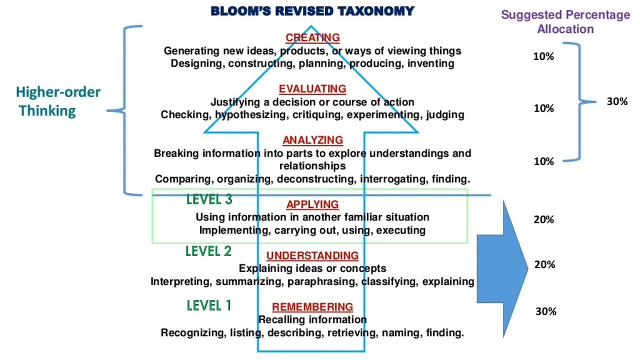 When the students implement, carry out, use and execute. That is applying For higher education. You measure students' understanding or their thinking skills, Which will fall under the average to difficult part. It is important that you know the domains Because you will classify your questions as to which domains they will fall. 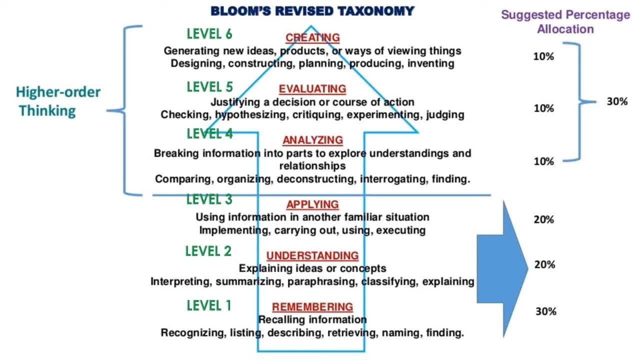 Now there is a suggested percentage allocation for each domain. Remembering, understanding and applying fall under easy to average and take up the 70% of the total test items. Analyzing to creating takes the 30% of the total test items. 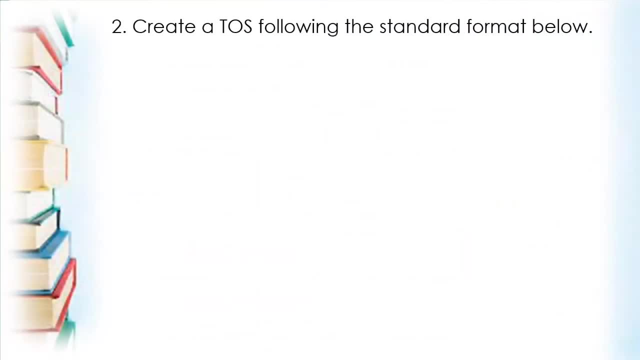 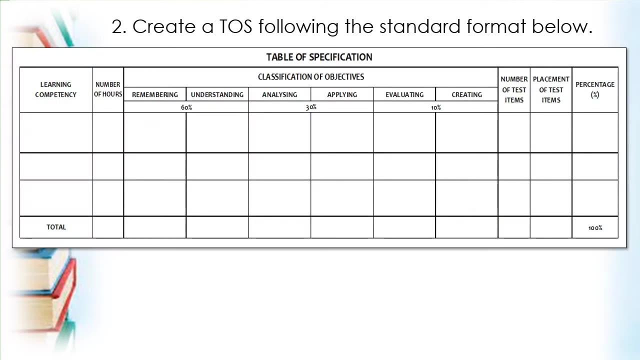 Second of the things you need to know is the creation of a TOS table following the standard format, This one. This is the standard format of DepEd. However, I innovated this one. It is simpler, but the salient parts have not been eliminated yet. 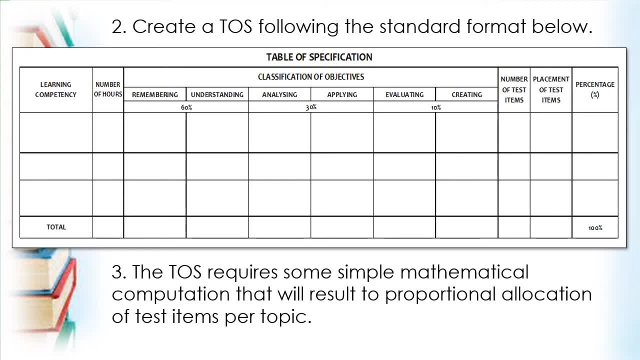 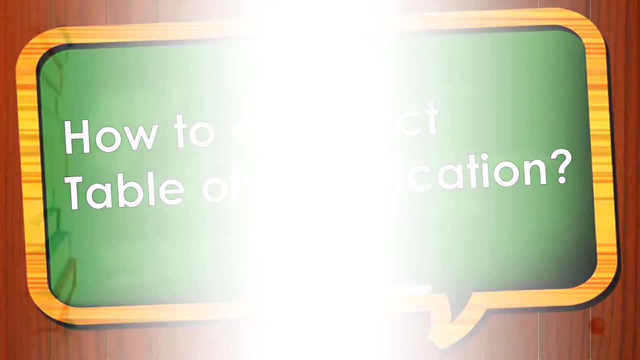 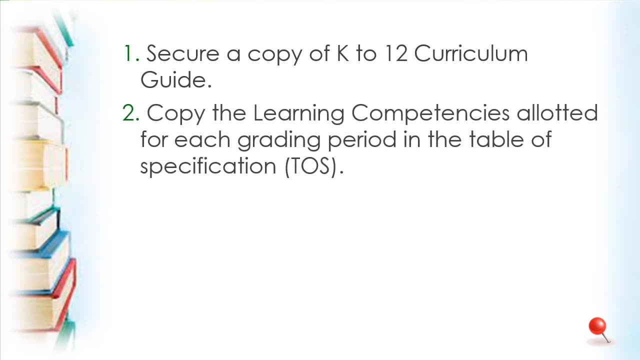 I'll show you later. And third, The TOS requires some simple mathematical computation that will result to proportional allocation of test items per topic. How to construct table of specification: First, secure a copy of K-12 curriculum guide And copy the learning competencies allotted for each grading period in the table of specification. 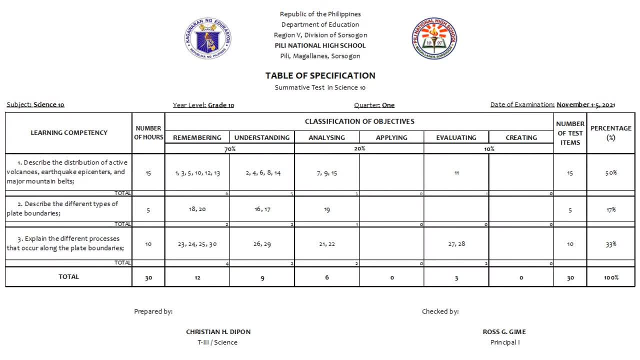 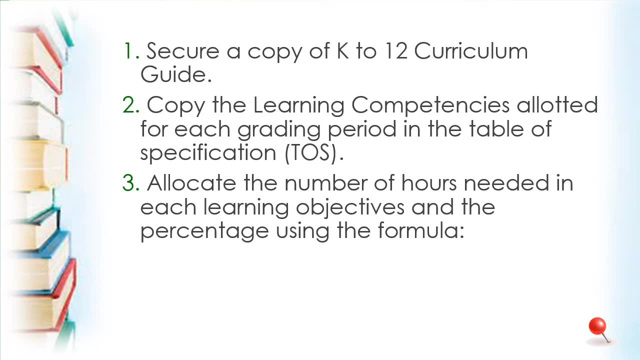 Like this one. This is the TOS I made for my grade 10 class, Science 10.. And here are the learning competencies that I achieved for quarter 1.. Third, Allocate the number of hours needed in each learning objectives And the percentage using the formula: 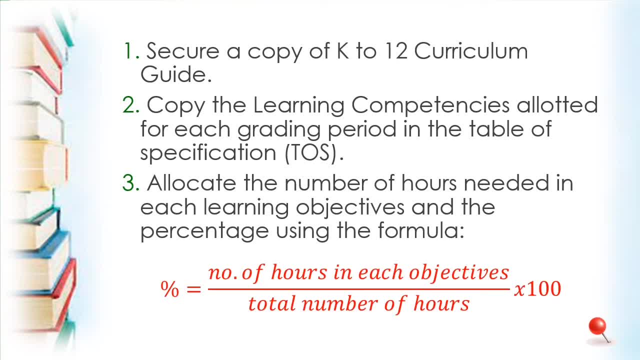 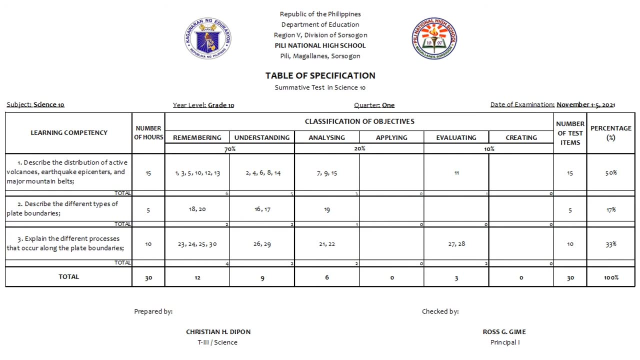 Percent equals number of hours in each objectives divided by the total number of hours times 100.. Like this, Learning competency number 1 was taught in 3 weeks And that is equivalent to 15 hours. Learning competency number 2 is 5 hours. 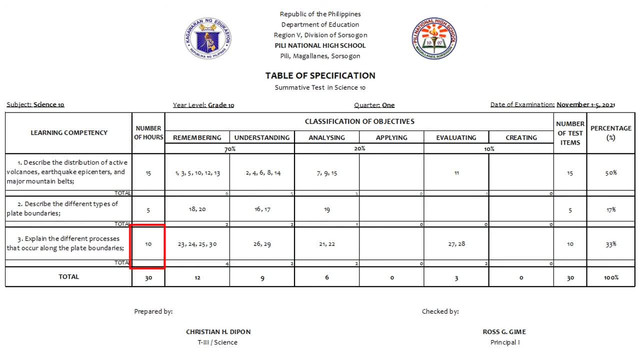 And learning. competency number 3 is 10 hours. So that is a total of 30 hours. Now to get the percentage value 15.. The number of hours Divided by the total number of hours Times 100. That is. 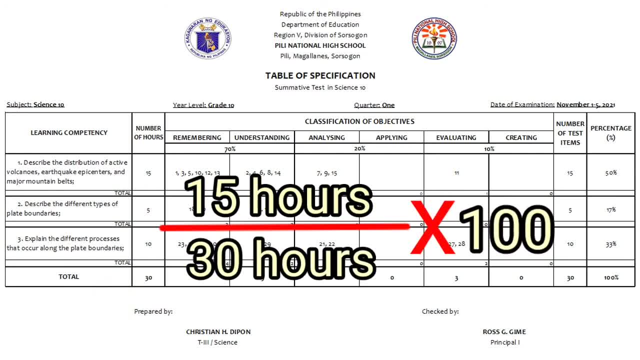 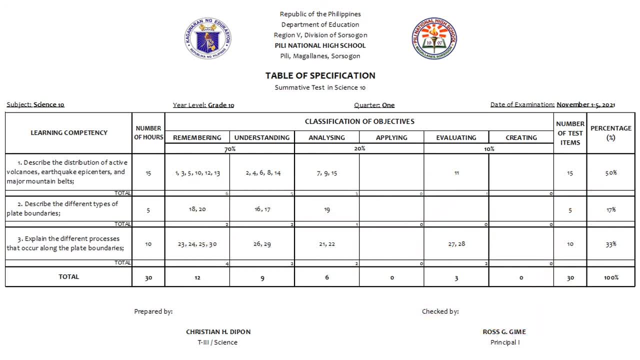 15. Times 100.. That is 50%. 15 divided by 30.. Times 100 is 50%. Learning competency: number 2.. 5 divided by 30.. That is 17% And 10 divided by 30.. 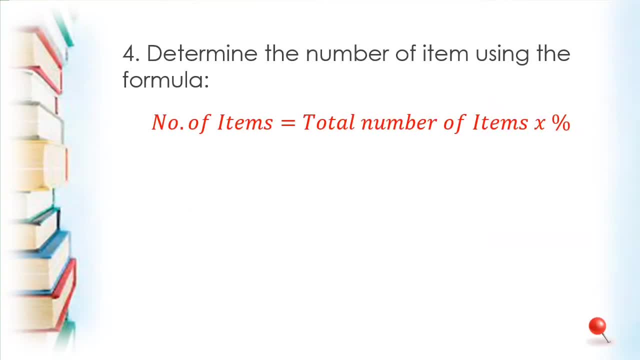 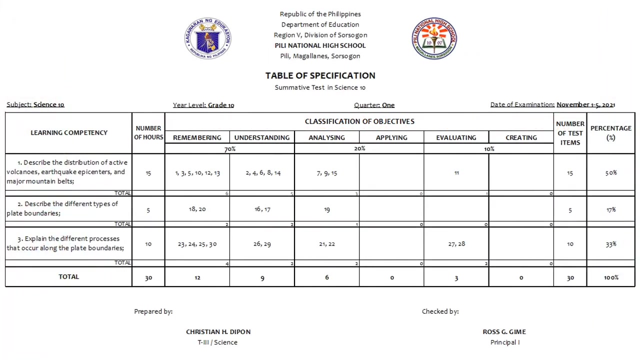 Is 33%. Fourth, Determine the number of items using the formula: Number of items equals total number of items times percent. Like this, Let's say, For learning competency number 1. We have 50% And The total number of test items. 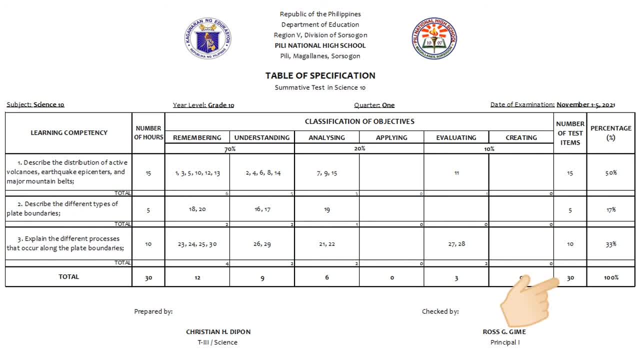 That we will do is 30. So 30. Times .50, Or the 50% of 30. Is 15.. So the number of test items Is 15. 30. Times .17, Or the 17% of 30.. 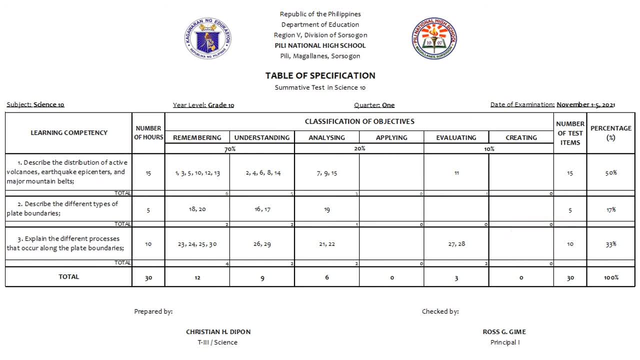 Is 5.. Learning competency number 2.. 5 items only For learning competency number 3.. 30 times .33, or 33% of 30. Is 10.. And that is the 30 item test That you will do. 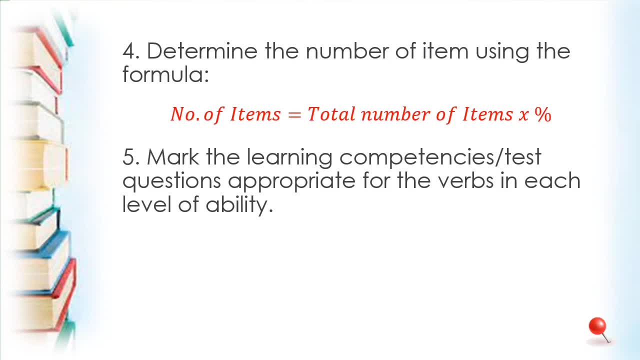 Fifth, Mark the learning competencies test questions Appropriate for the verbs In each level of ability And, after marking, Allocate the number of test items For each topic In each classification of objectives. Follow the 60,, 30, 10% format. 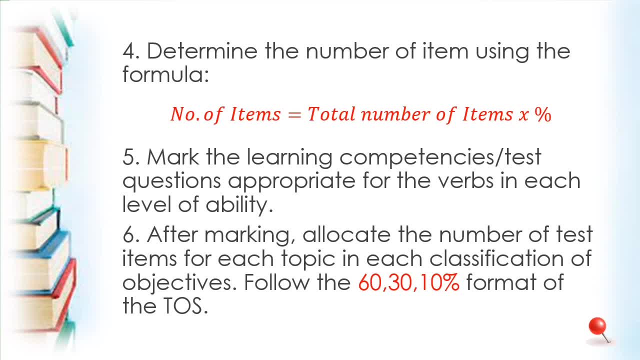 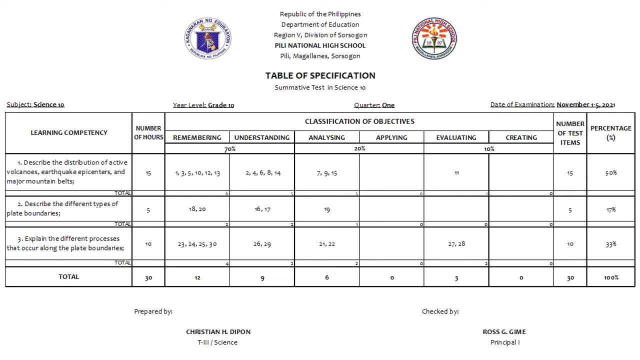 Of the TOS Like this. So when you have done the test questions For learning competency, You will allocate Where the domains Or classification of objectives Will fall Under: remembering, Understanding, Analyzing, Applying, Evaluating And creating.